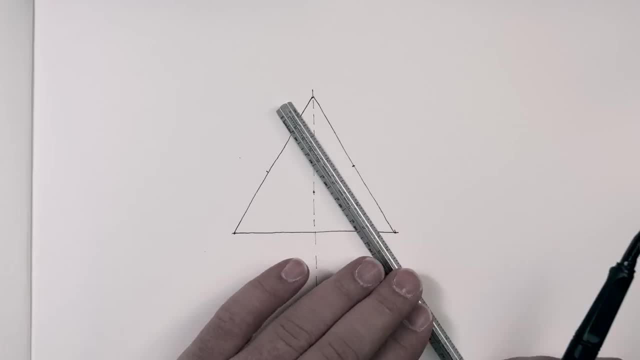 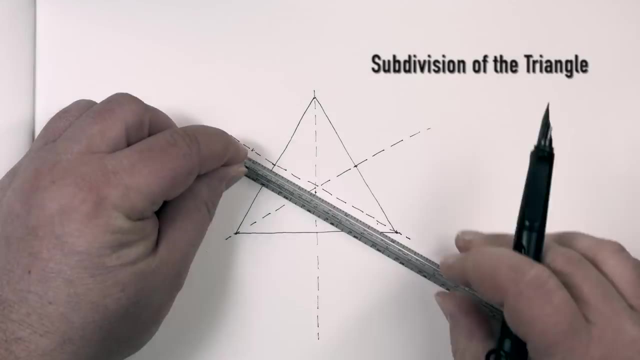 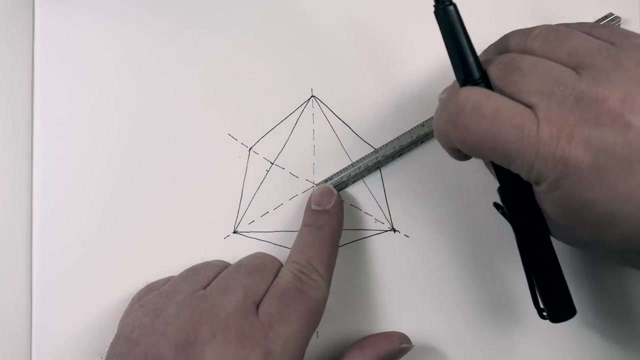 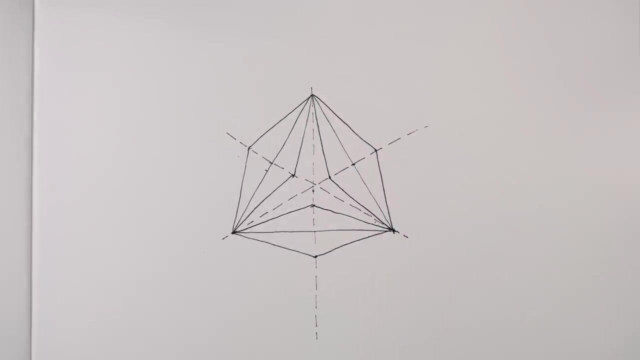 but he also taught him a philosophy of architecture that would stay with Frank Lloyd Wright throughout his career. He uses the subdivision of a triangle, sometimes called formal subdivision or dynamic symmetry. Sullivan was often called the father of the skyscraper and the father of modernism, and was a mentor to Frank Lloyd Wright. He was the first. 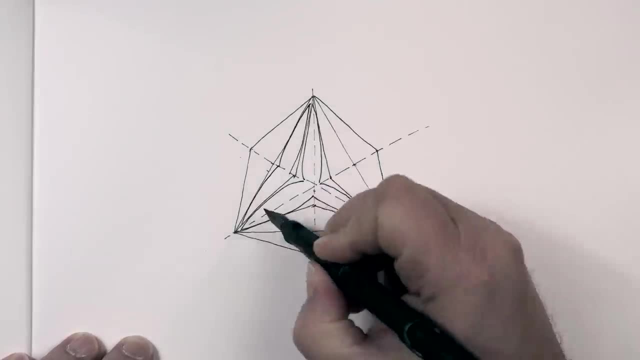 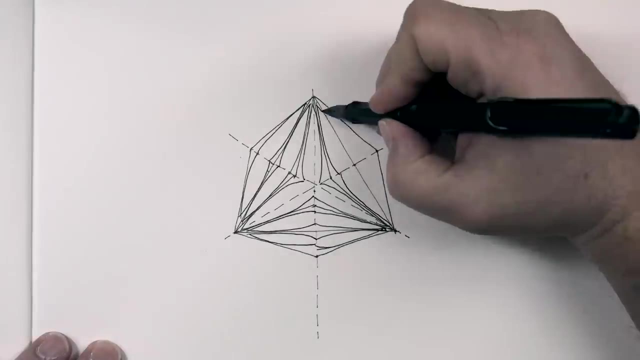 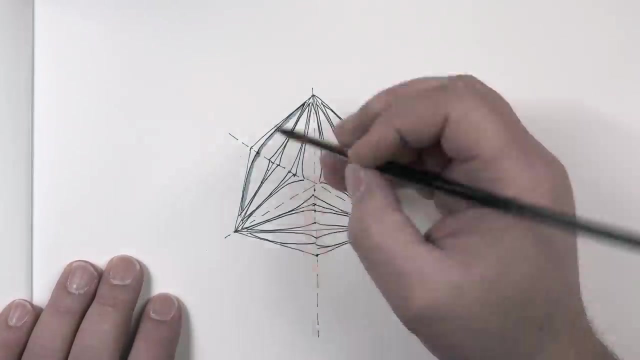 architect. to use the term, form follows function, but his idea was a more organic conception of nature rather than the German functionalist one. at the time, Sullivan worked for the great American architect, Frank Furness, before moving to Chicago and being part of the Chicago School. 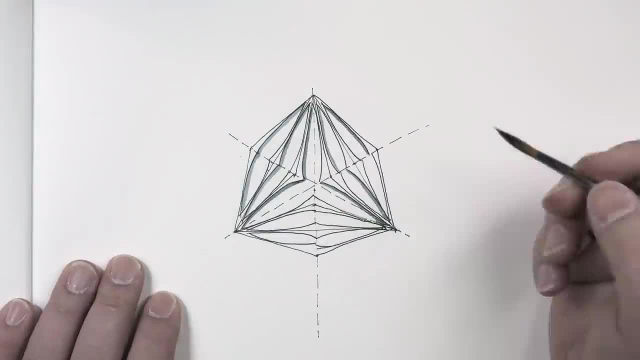 of Architecture, Wright called Sullivan Liebermeister, suggesting that Sullivan was his artistic inspiration. Frank Lloyd Wright was the first architect to use the term form follows function, but his idea was a more organic conception of nature. rather than the German school of architecture, Sullivan is a very artistic mentor in architecture and design. 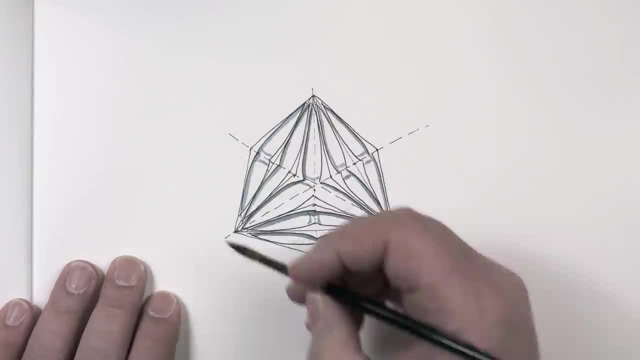 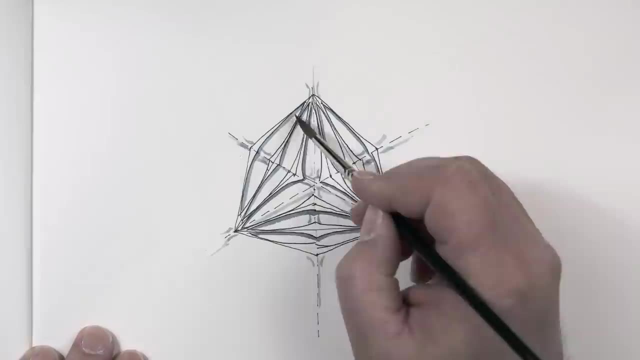 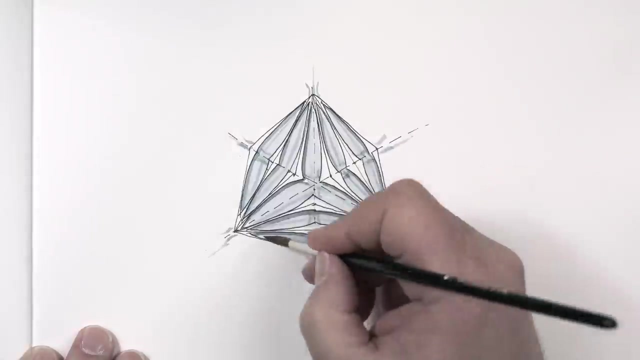 It seems that Wright copied Sullivan's geometric design process almost exactly. What Wright worked out, taking Sullivan's process to the next level, was to take formal geometric subdivision from two dimensions in the ground plane to three dimensions to create architectural space. This process was used in 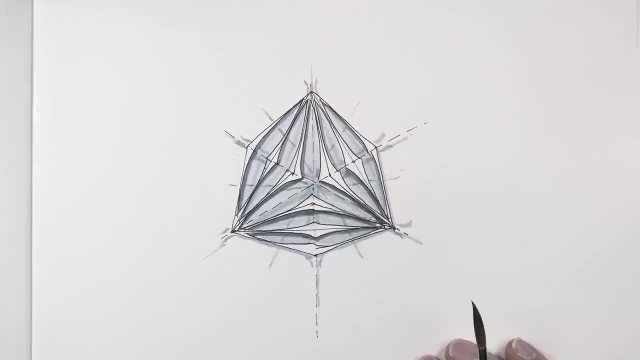 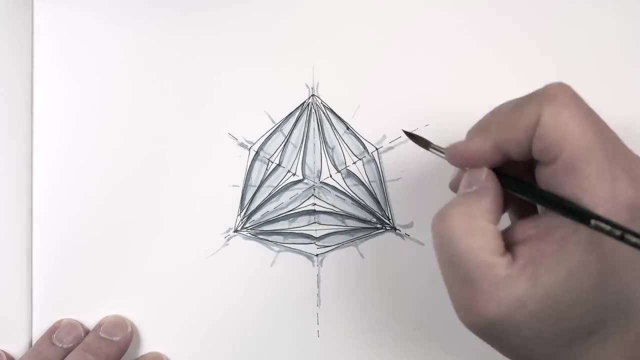 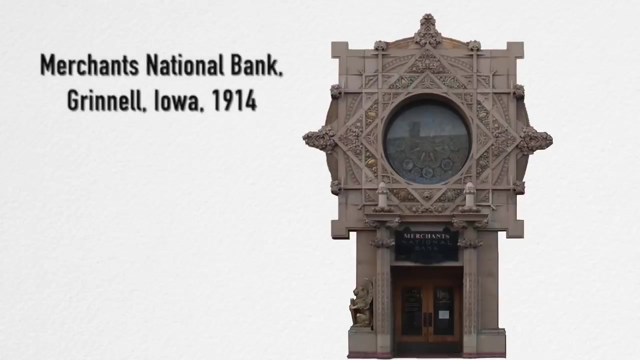 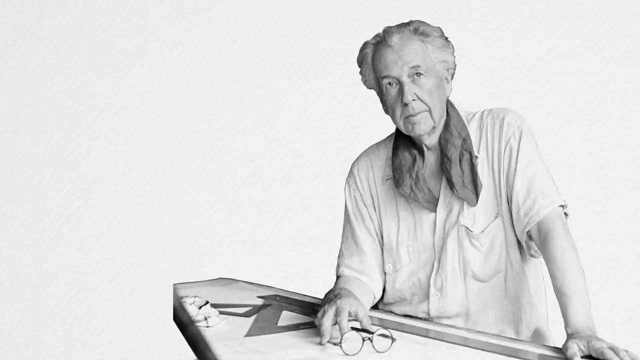 formal design in Renaissance architecture, but Wright's use of it was unique and based more on Sullivan's art style. Here we see one of Sullivan's designs on the Merchant National Bank in Grinnell, Iowa, from 1914.. Frank Lloyd Wright used several principles in his work, including starting with geometry. 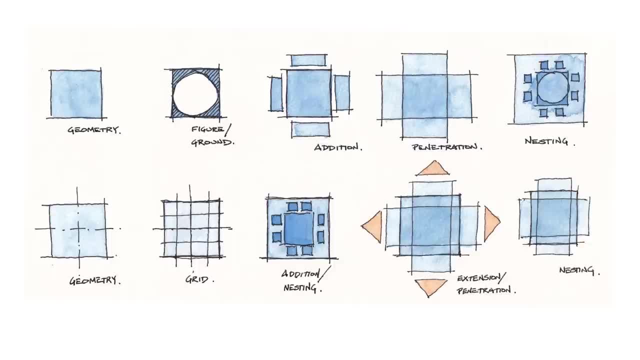 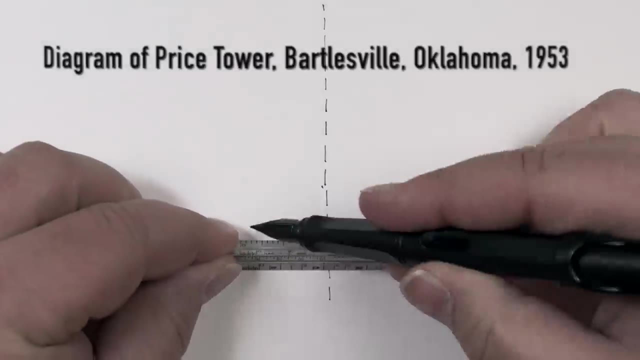 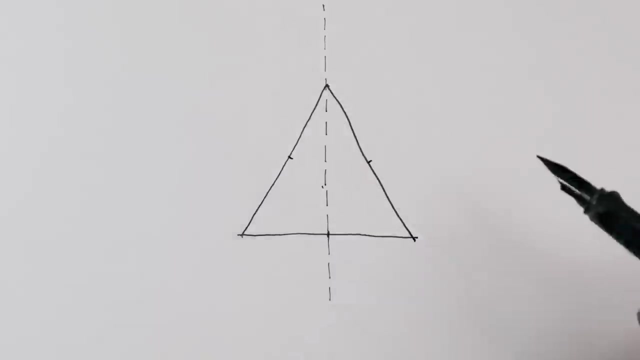 figure: ground, addition, penetration, nesting a grid: addition, extension or penetration and nesting. Sullivan states in his book A System of Architectural Ornament: These simple forms of ancient discovery and use were given esoteric meanings and occult powers by the men of that day in an effort to create a system of architectural ornament. 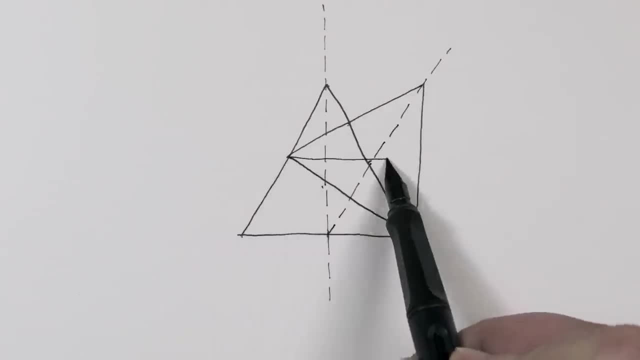 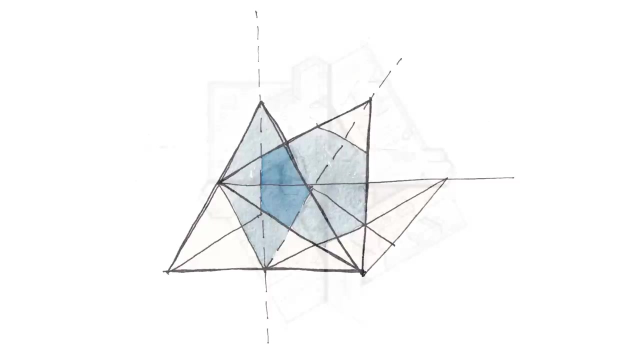 In an effort to control, by means of formulas and secret rituals, the destiny of man amidst the powers of nature. With mystic numbers and other phenomena, they formed part of an elaborate system of magic to which the world penned its faith. This is a diagram of Price Tower in Bartlesville, Oklahoma. 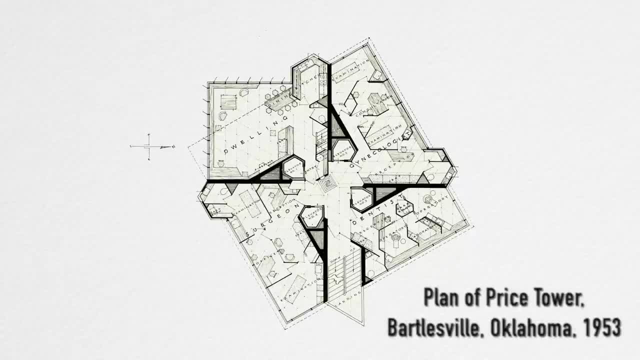 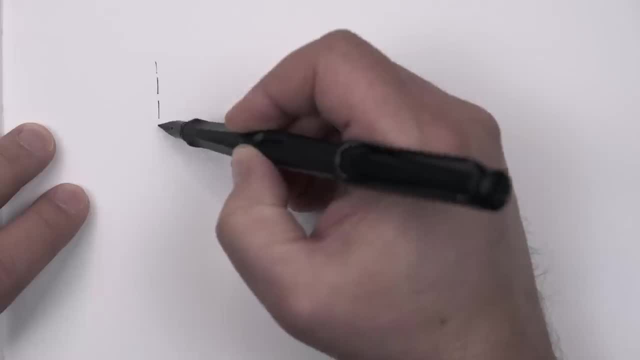 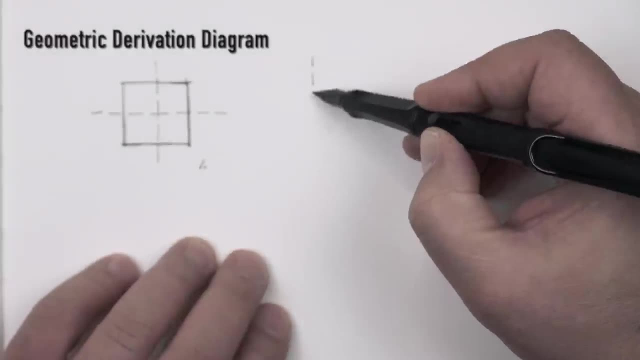 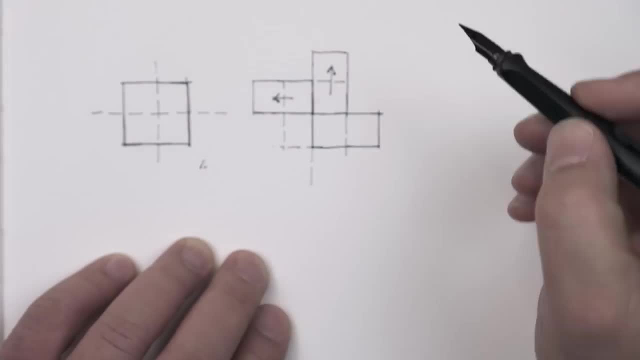 from 1902.. One technique Frank Lloyd Wright was particularly fond of was the pinwheel. This was a technique he used in his work on the pinwheel. The pinwheel is the longest wheel on a train and the most popular one is the pinwheel. 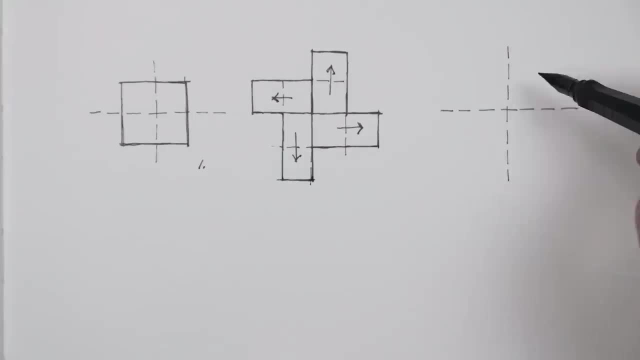 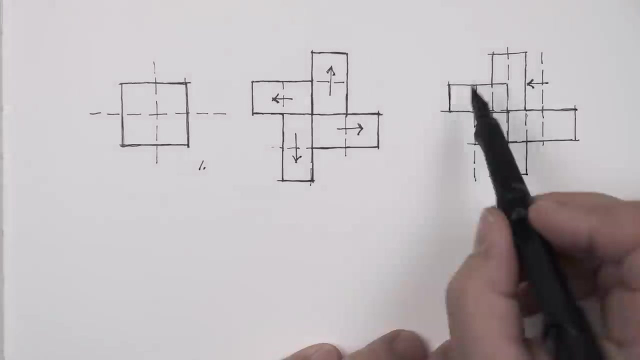 the pinwheel of the pinwheel, where he would take a geometric form and have it rotate around a center, creating a pinwheel-like effect. Then, once the pinwheel was created, he would move and manipulate the different forms from the pinwheel. 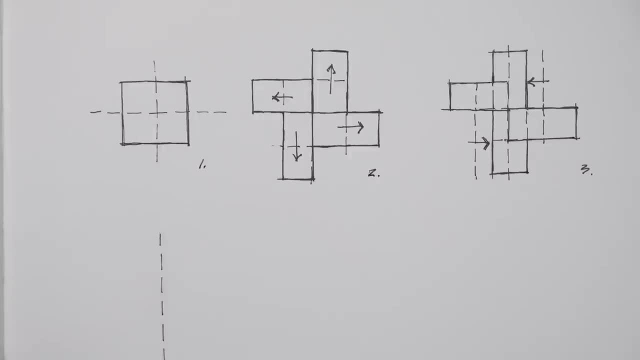 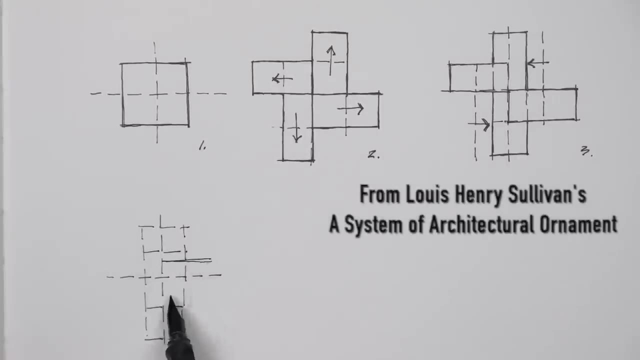 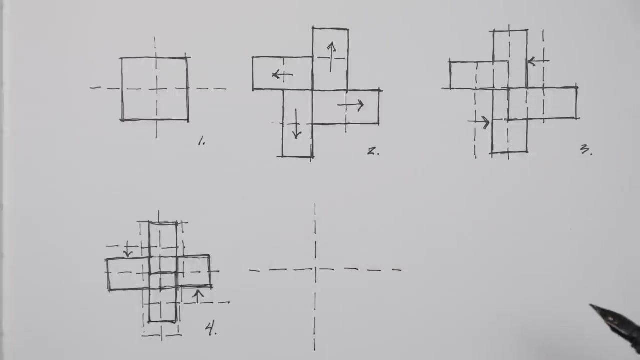 This is done by rotating a form around a center. Technically, as an item in the progress of our demonstration, the above forms, rigid in their quality, are to be considered in our philosophy as containers of radial energy, extensive and intensive, that is to say, extensions of form along lines or axes rating from the center. 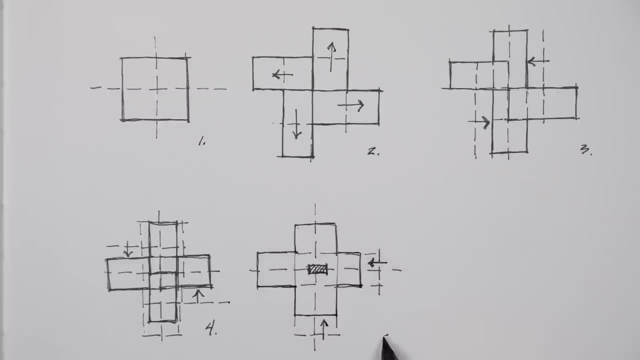 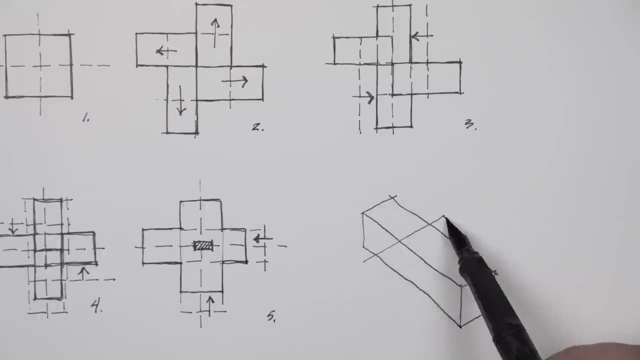 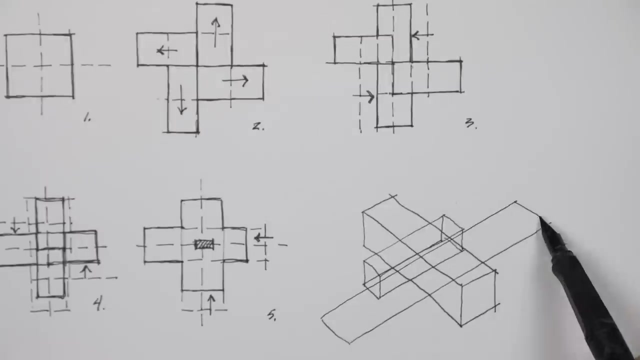 and intentions of form along the same or opposite axis. Here then appears the will of man to cause the inorganic and rigid to become fluent through his powers. Also, note that we assume energy to be resident in the periphery and that all lines are energy lines, and this may be called plastic geometry.